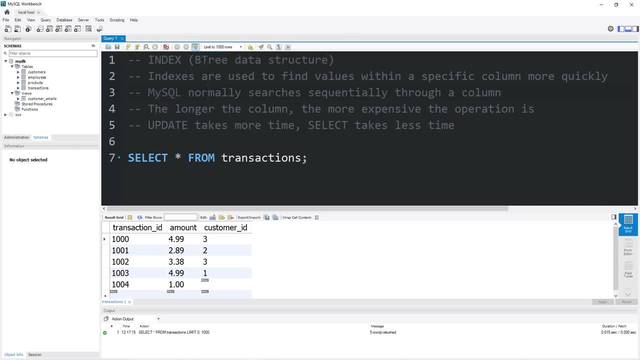 is, but if you don't, don't worry about it. MySQL normally performs searches sequentially through a column. If I'm looking for some specific value, I can just scan each value on the way down to see if those values match depending on what I'm looking for. It doesn't really take much time. 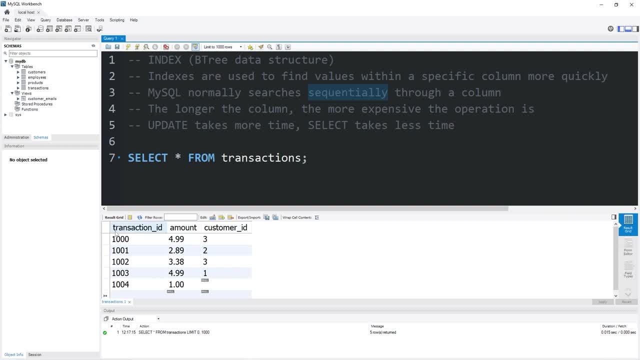 if you have a small data set, like I do, but imagine if you have millions of transactions. Searching each transaction one by one is going to take a long time. We can speed up that process by using an index. By applying an index to a column, selecting or searching takes less time. However. 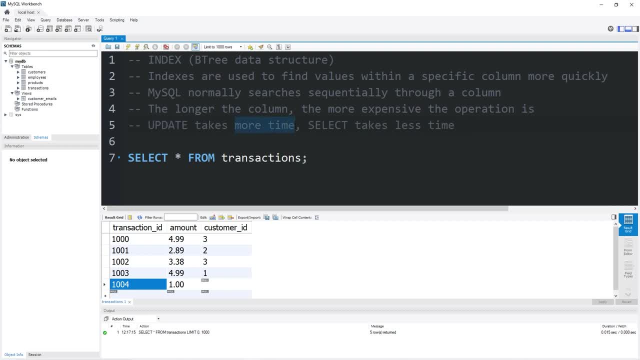 updating takes a lot more time. So there are some pros and cons with using an index. It really depends on the table. If I'm working with a table of transactions, transactions are being updated all the time. People are constantly making purchases. I don't think our transactions table would. 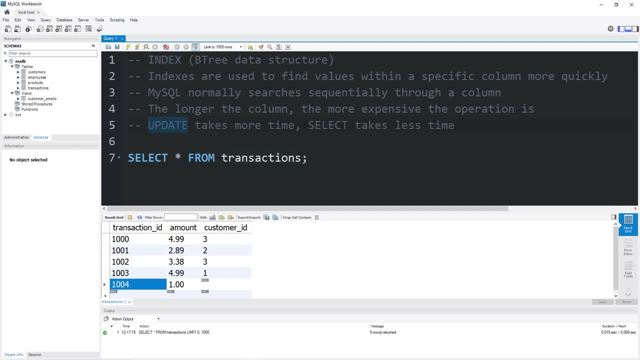 be a good candidate for an index. We'll be doing a lot of updating but not a lot of searching. However, with our customers table, I think our customers table could benefit. We don't update our customers table very often. Only a new customer comes in every once in a while. 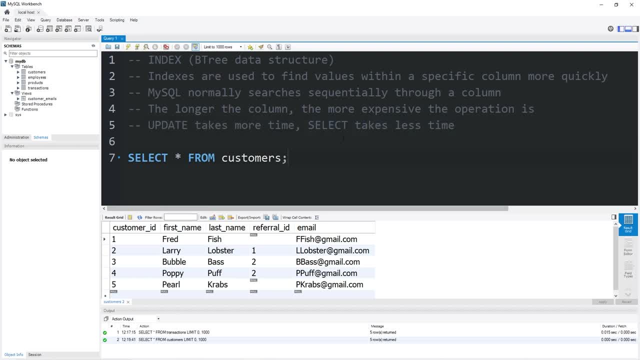 Let's reduce the time it takes to search for a customer With creating an index. how exactly do we want it to be? We want to find the customer, Believe it or not. we do have an index with our customer ID already. A customer may give you their last name and or first name. 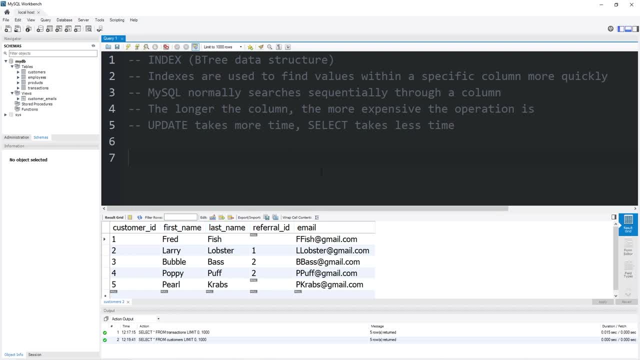 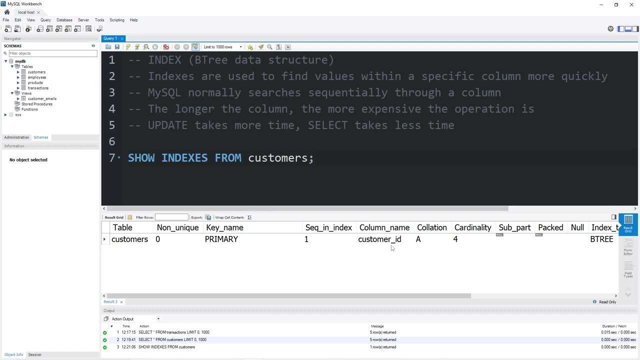 Let's create an index for these. We'll start with last name, though. To show the current indexes of a table, you would type: show indexes from the name of the table. Here are the current indexes for our customers table. We do have one already and that's for our customer ID. That is the primary key. 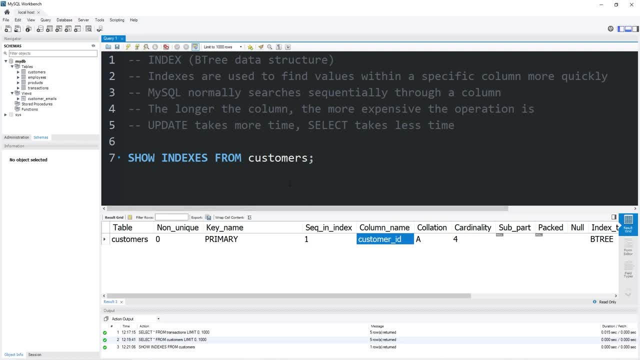 Let's search for a customer by their customer ID fairly quickly, but not so much by their last name or their first name. Let's apply an index to those columns. To create an index, you would type create index, then a name. I will apply an index to our last name column. I will name this index last name, IDX, meaning index. 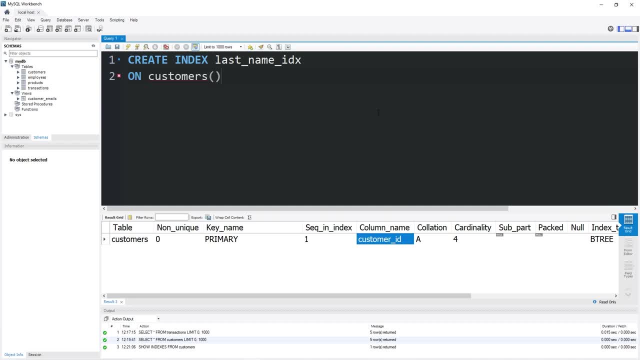 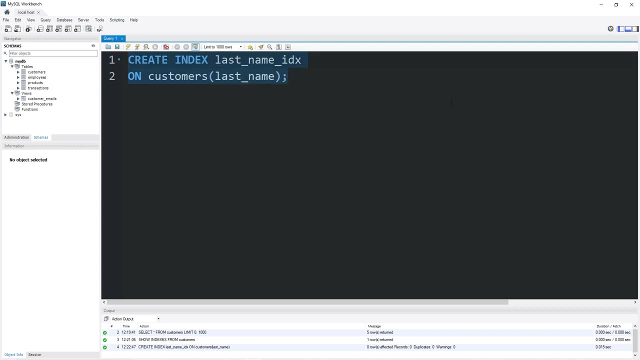 On the table- customers in this case- then list a column. I will apply an index to our last name. We will be doing a lot of searching by a customer's last name, so I might as well apply an index. So let's execute the statement. Let's show our indexes again. 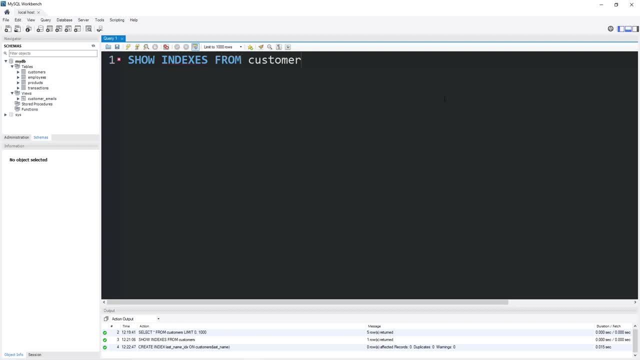 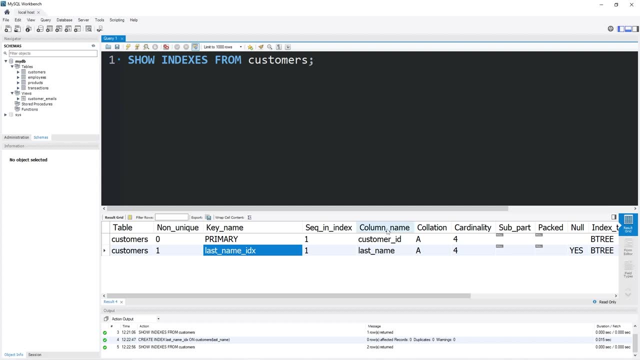 Show indexes from customers. And here is our new index: Last name index. It's applied to our column last name. If I were to search for a customer by last name, that process will be sped up now. Select all from customers where last name is equal to puff. 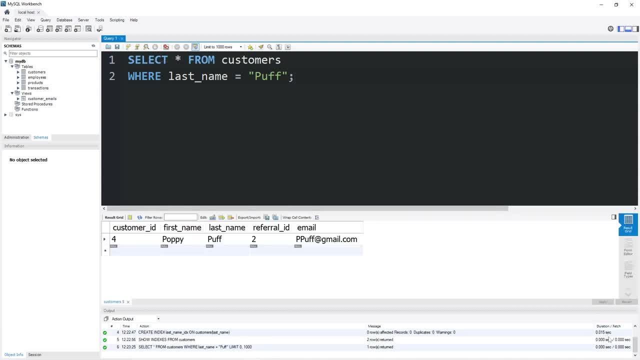 So my data set is already very small. to begin with, There's not going to be a noticeable difference in this example, but if I'm working with a million customers, using an index would be a lot faster If I were to search by first name instead. 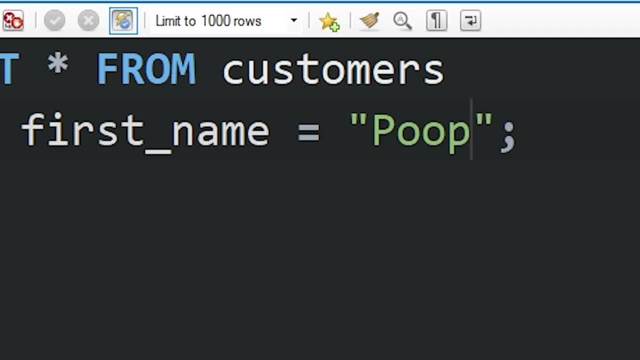 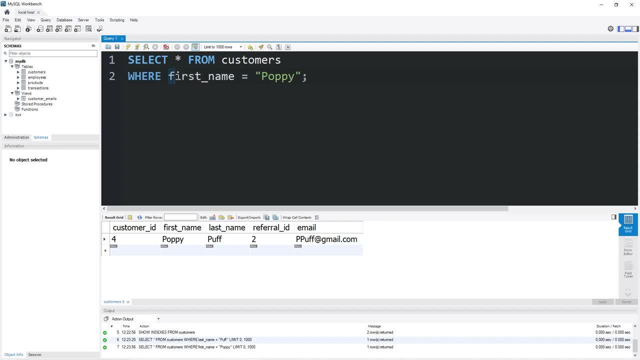 where first name equals poppy. uh, I spelt poppy wrong. Well, we don't have an index, so we're going to use indexapplied to our first name As of now. it would be slower to search for a customer. 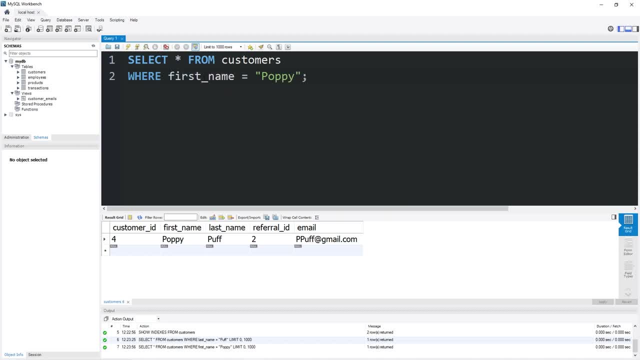 by their first name compared to their last name. That first name doesn't have an index. Realistically we wouldn't search for a customer just by their first name. We would do a last name or a last name and a first name. 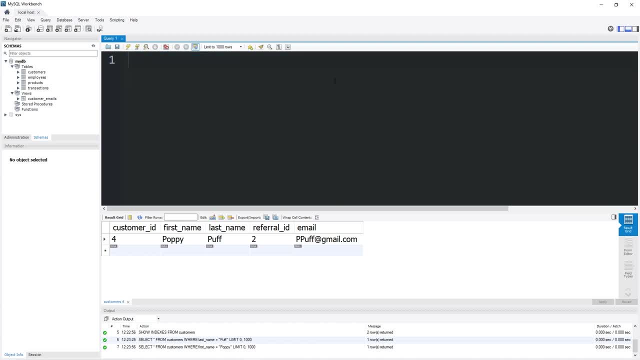 That's where multi-column indexes come in. To create a multi-column index you would type create, index a unique name, let's say last name, first name, idx- on our table. customers then list the columns in order. The order is very. 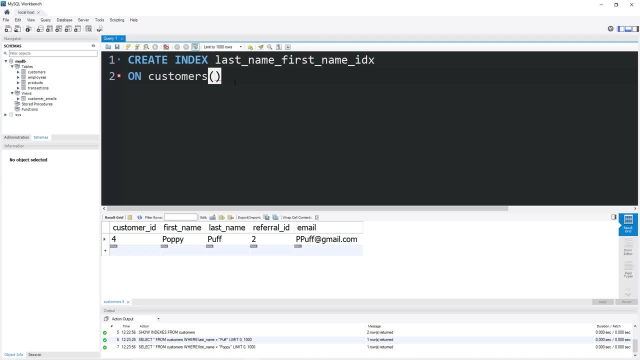 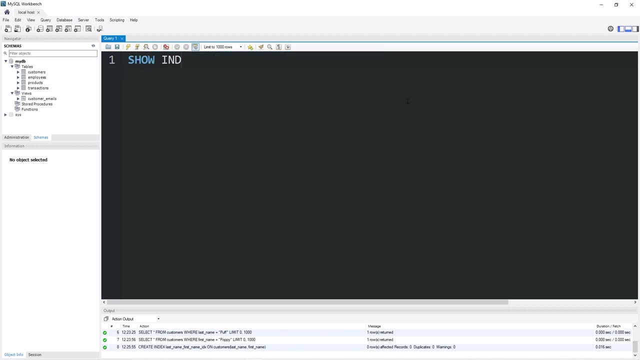 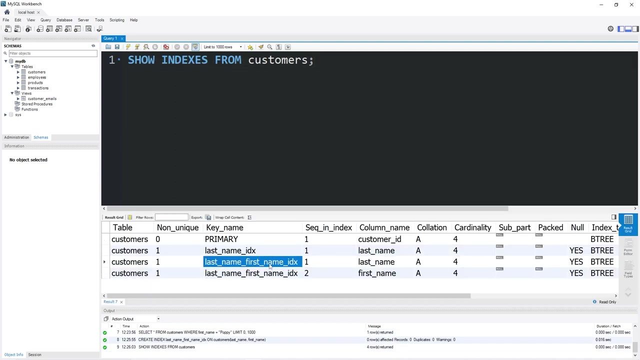 important. MySQL has what's known as a leftmost prefix with indexes, so we will search by last name, then first name. Let's execute the statement: Show our indexes. Show indexes from customers. Here's our last name, first name, index. There's a sequence We're telling. 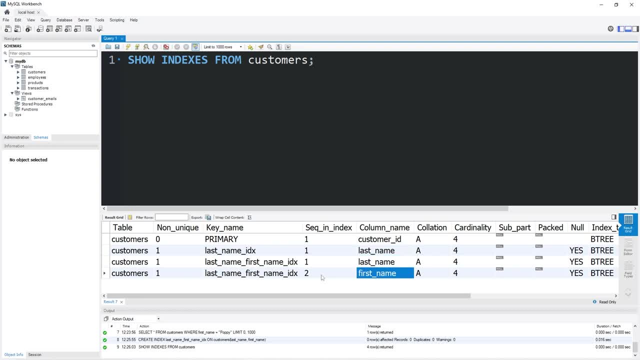 MySQL to search by a last name. However, if there's also a first name, include that too. There needs to be a last name to utilize this index. If I want to, I can get rid of this last name index, because our last name, first name index would do the same thing. We can search.